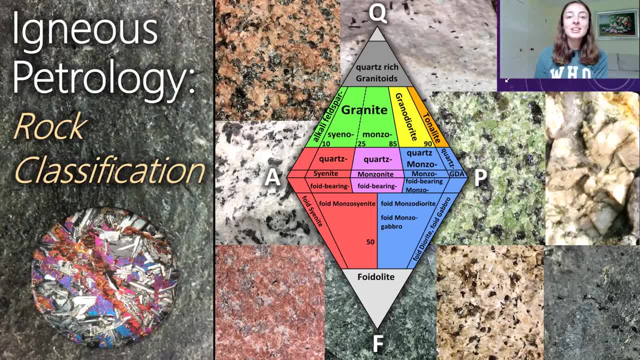 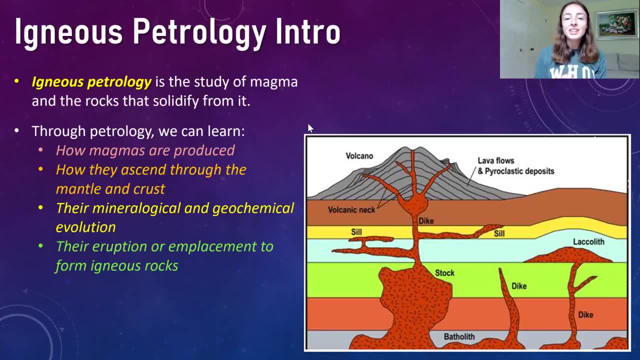 hey guys, today we're going to be talking about igneous rock classification, so let's get started first, because this is the first lecture i'm doing over igneous petrology, i just want to give a little bit of background into what igneous petrology is or what it means. so, basically, 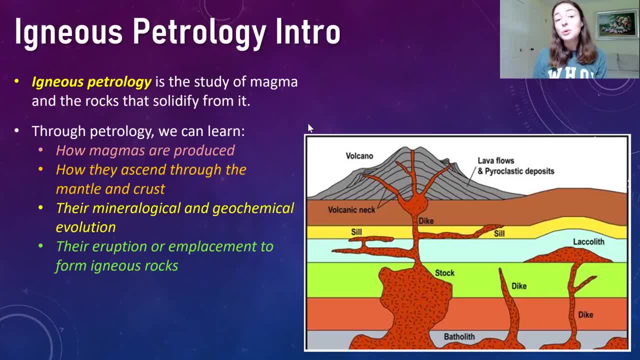 igneous petrology is the study of magma and the rocks that form from it or that solidify from it, and through studying igneous petrology we can learn a lot of different things, for example, how magmas are produced, how they ascend through the mantle and crust, their neurological and 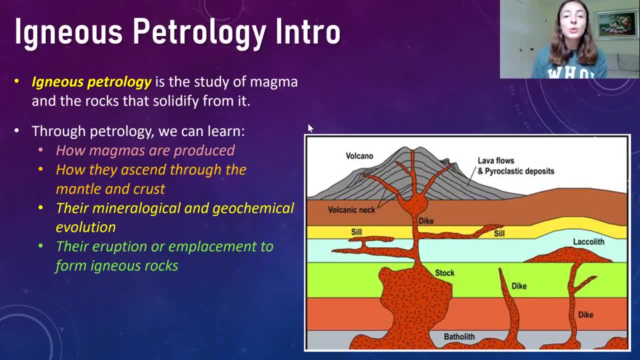 geochemical evolution and their eruption or emplacement to form igneous rocks. so we'll be talking about all of these things in this igneous petrology playlist. so be sure to stick around for all the videos to get all of this information. but before i jump right in, i want to 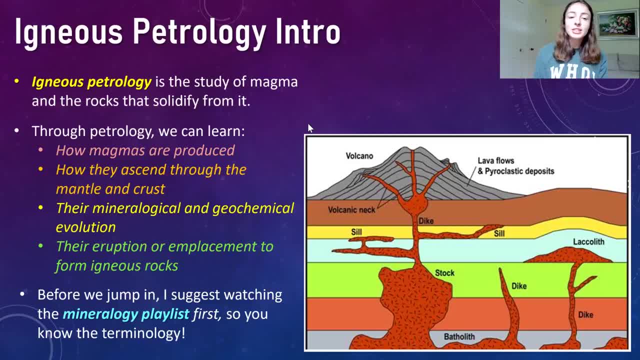 warn you that a lot of the terminology that we use in igneous petrology is the same as what we defined in the mineralogy videos, and i have a mineralogy playlist if you want to go check that out first, because that will really help you to understand a lot of the things that 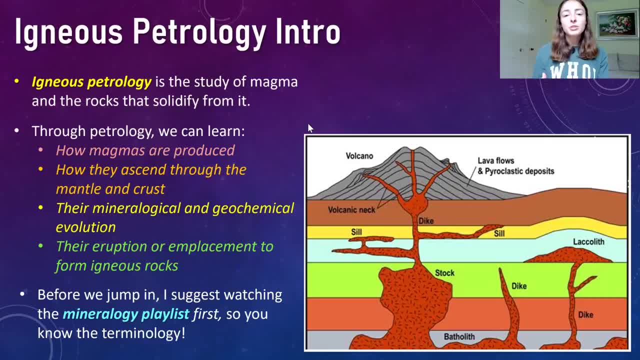 we are talking about in this playlist. now i will try my best to go back and redefine a lot of the terms, but if there's anything you don't understand, be sure to go check those videos out over mineralogy to kind of get yourself acclimated to the terminology that we use in igneous petrology. 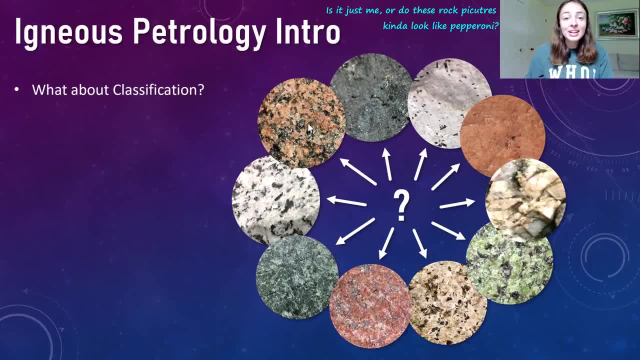 so what about classification? this is the topic of this video, right? yes, so let's go over how we can classify igneous rocks. there are a lot of different ways to classify igneous rocks. i'm going to talk about a few main ways that we classify igneous rocks in. 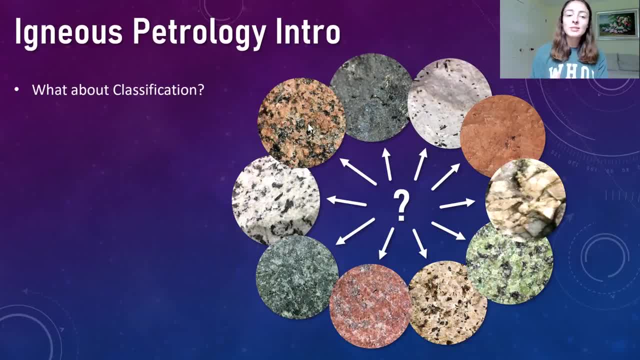 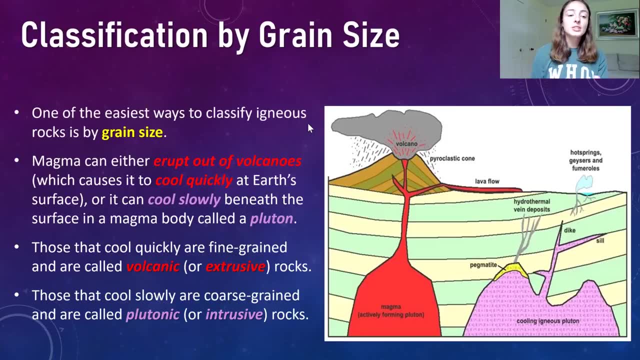 this lecture, however, i'm going to start with the most broad or easy classification system, and that is classifying by grain size. so before we can talk about the classifications by grain size, though, we need to talk about how igneous rocks form with different grain sizes, so there are two main ways. 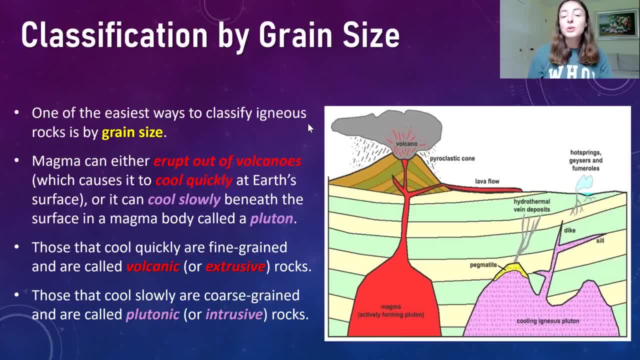 igneous rocks. it can either erupt out of a volcano and cool quickly at earth's surface to form igneous rocks, or it can cool slowly within a pluton below the surface of earth, and so we can see that in this figure to the right. here we have this red magma body that is shooting up, ascending. 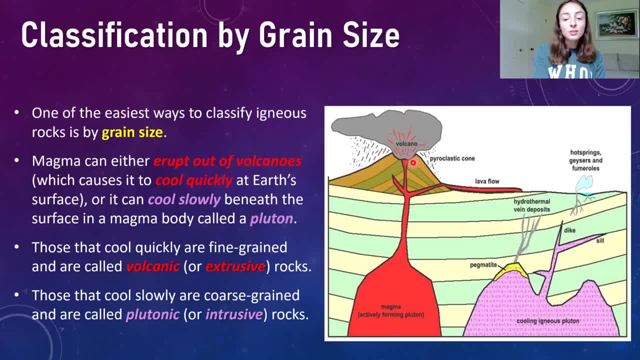 through earth's crust to get to this volcano at earth's surface. then it explodes out of the volcano and some of it comes over here and does a lava flow, and so you've got this exploded material that's cooling extremely quickly, and then you've got this flow that's cooling extremely quickly. 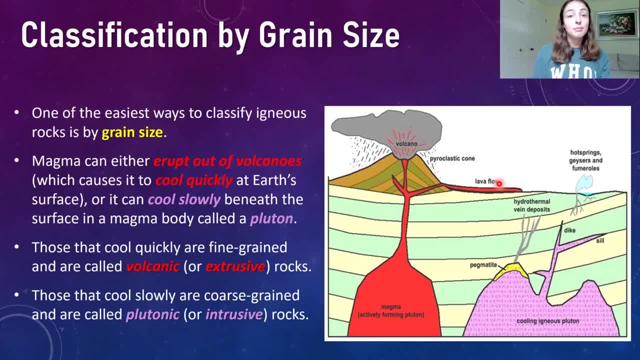 as well, because it's going from a hot environment to a much cooler environment very quickly, whereas you have this pluton over here to the right. that is, this magma body within the earth that's cooling, but at a much slower rate because it's not actually reaching the surface of earth to cool. 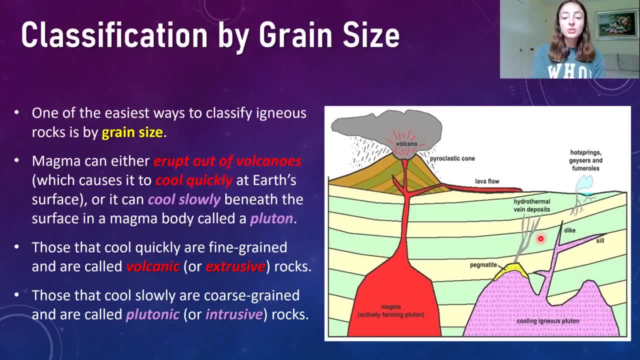 so we have a classification system in which we call these two different methods of cooling rocks to different names. so what we call the ones that explode out of a volcano is a volcanic, which is aptly named, or extrusive, because it's exiting the earth, but we call these ones that cool below. 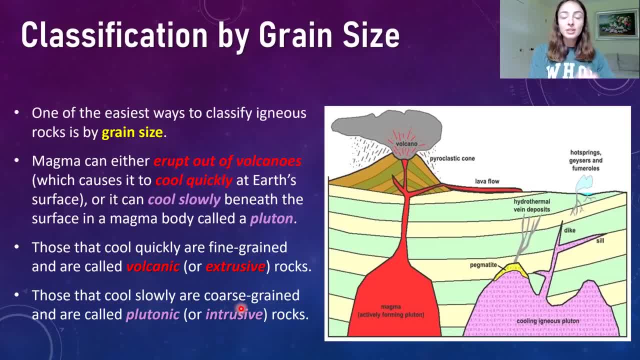 the surface of earth. intrusive, because it's within the earth, it's not exiting. or plutonic, which makes sense because they're cooling in a pluton. so these names are pretty easy to remember, thankfully because we know that science doesn't always give us easy names to remember. so 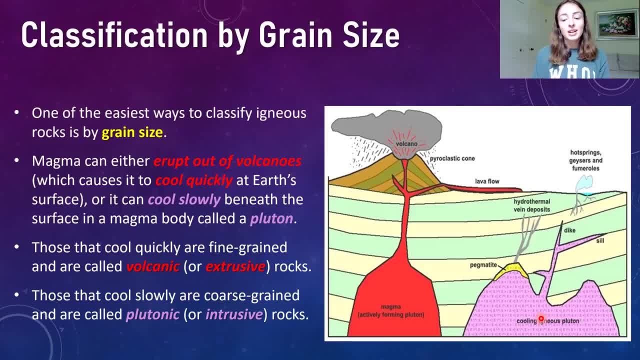 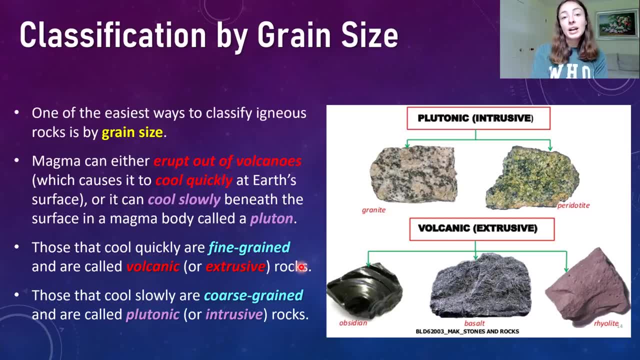 then the question is: what the heck does this have to do with grain size? well, it's pretty simple. basically, the rocks that cool quickly, or volcanic or extrusive rocks- are very fine grains. so they have very tiny, tiny grains or no grains at all if they end up being glass. 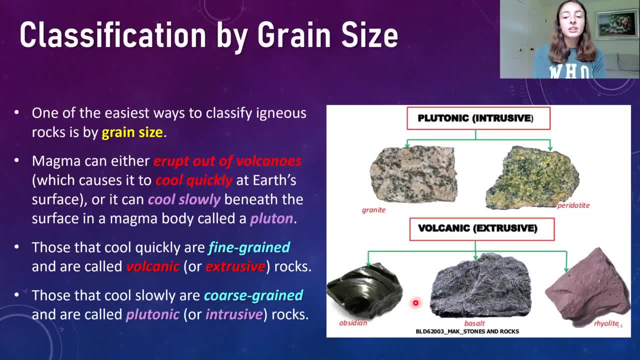 glass only happens if it cools like instantly, and then you get these finer grained rocks that also cool very quickly, but not as quickly as glass. so you have fine grain, extrusive or volcanic rocks, but the ones that cool slowly end up being coarse grained. these are plutonic or intrusive rocks. so 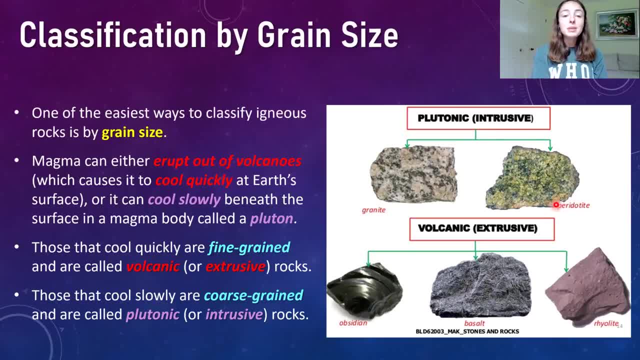 you get these coarse grains in these rocks because when the magma is allowed more time to cool, it allows those crystal grains more time to grow, whereas when the magma cools quickly, it doesn't allow those crystal grains that much time to grow. so you get fine grain rocks and we'll talk about. 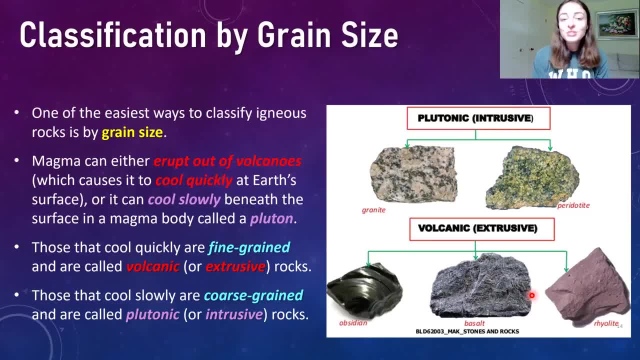 this a lot more in the upcoming igneous rock textures video, so look out for that if you want to know more about why grains can become coarse or why they become fine and how crystal nucleation and growth rates all affect this. so we'll talk about that in that video if you want to check. 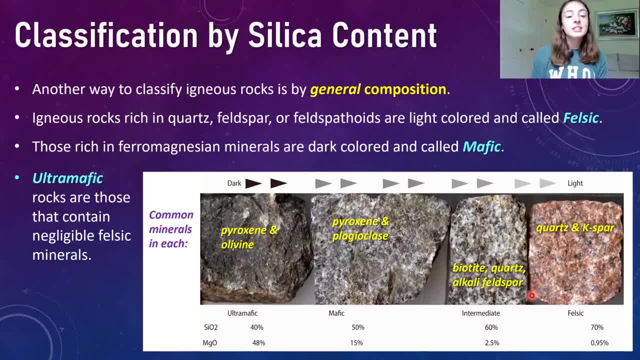 that out. but in this lecture we're moving on to the next classification method. this one is another broad classification scheme, so it's basically classified in these rocks based on their general composition or in this case, silica content, so igneous rocks rich in quartz, feldspar and 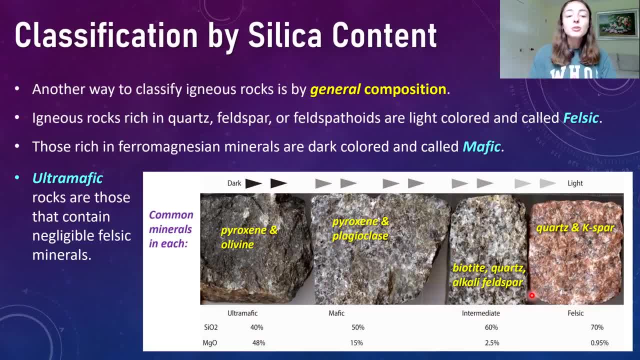 feldsploits are light in color and are called felsic, and those rich in ferromagnesian minerals, iron and magnesium minerals are dark in color and are called mafic, and the word felsic just comes from feldspar and silica and the word mafic. 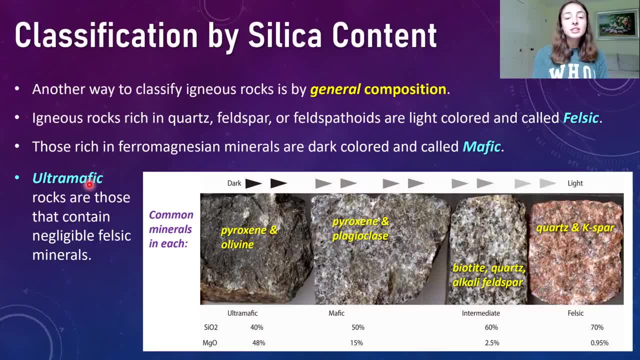 just comes from magnesium and iron. so if we look down at this figure, we see that light colored quartz and case bar ridge rocks are felsic. and then you've got intermediate here, because you've got quartz and alkali feldspar but you've got biotite, which is more of a mafic mineral. so this 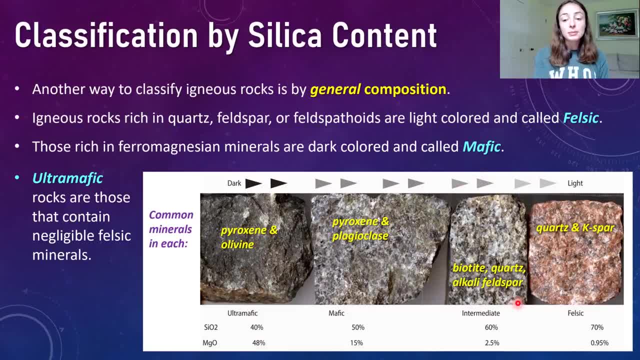 is intermediate and you can see, with the intermediate composition it's also intermediate in color. it's kind of between being very light and being darker, and then you have this darker one with pyroxenes and plagioclades and this is mafic, and then you have this really dark one which is termed ultra. 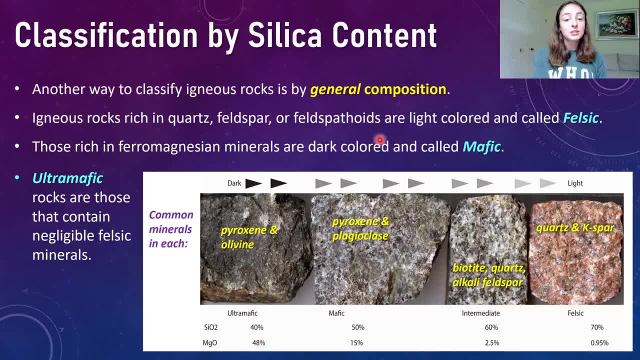 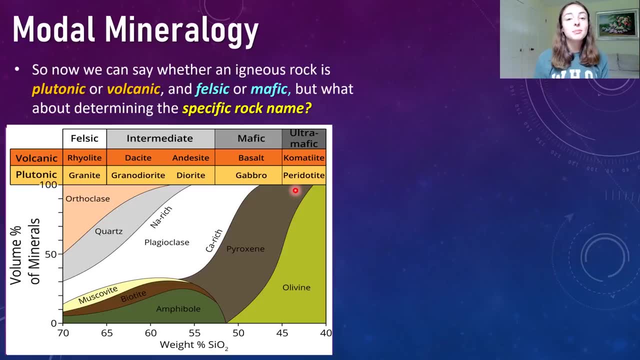 mafic, which are rocks that contain negligible felsic minerals, so hardly any quartz, feldspar or feldspathoids, if any at all, and ultra mafic rocks tend to have over 90 mafic minerals, such as pyroxenes and olivine. so now that we know how to classify an igneous rock based on its grain. 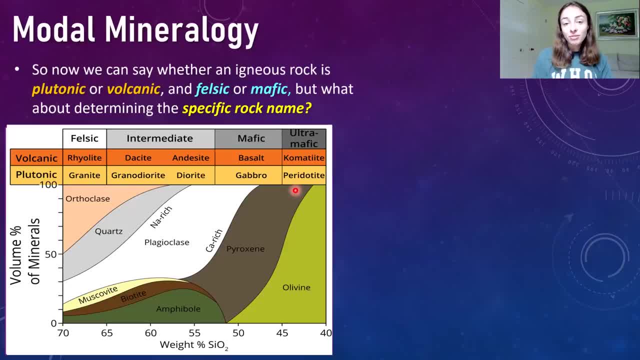 size- whether it's plutonic coarse-grained or volcanic fine-grained- and based on its color, whether it's light colored or felsic, or dark colored or mafic. but what about determining a rock specific name? because you likely have to do this in class and i haven't given you that yet. so first, 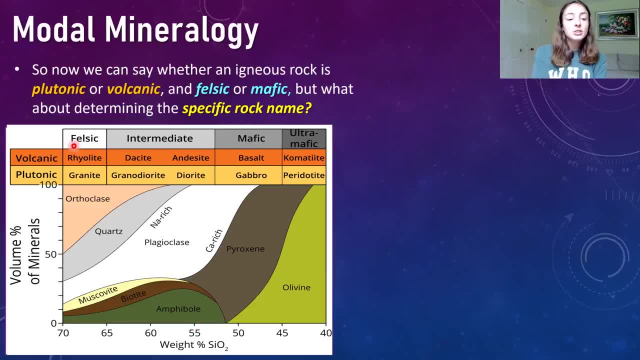 we can look at graphs such as this one down here on the bottom left, showing a felsic intermediate, mafic, ultra mafic transition of pyroxenes and pyroxenes. and then we can look at graphs such as this one down here on the bottom left showing a felsic intermediate, mafic, ultra mafic transition of. 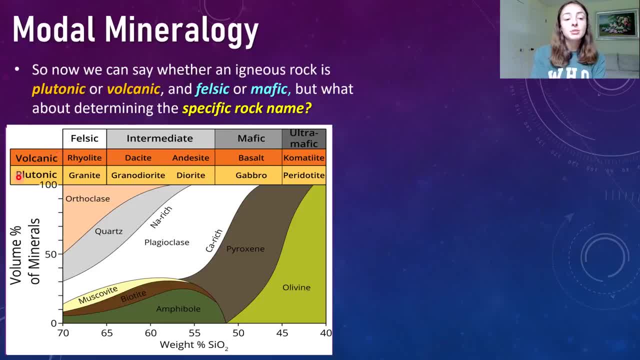 here from left to right and showing volcanic and plutonic over here on the left, and so we have volcanic refined grain rocks such as rhyolite in the felsic zone, daysite and andesite in the intermediate zone, basalt in the mafic zone, comatite in the ultra mafic zone, and then we 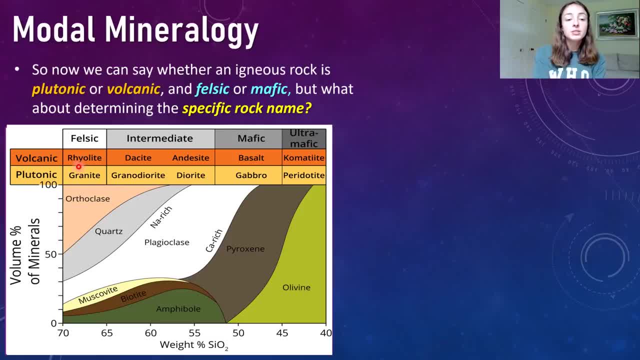 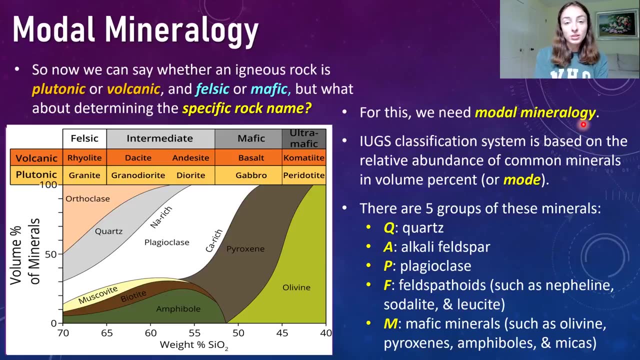 have their plutonic or coarse-grained equivalents, such as the felsic granite, the intermediate granite, diorite and diorite, the mafic gabbro and the ultra mafic peridotite. however, how did we arrive at these names? well, for that we need something called modal mineralogy, and 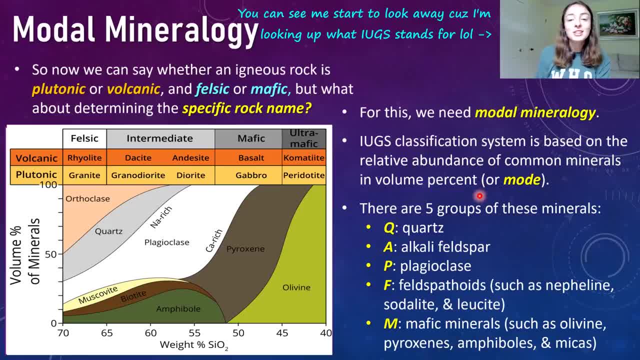 what this means is basically that the iugs, or international union of geological sciences, invented a classification system based on relative abundance of common minerals in volume, percent or mode, and that's why it's called modal mineralogy, because we're taking the mode or volume percent of 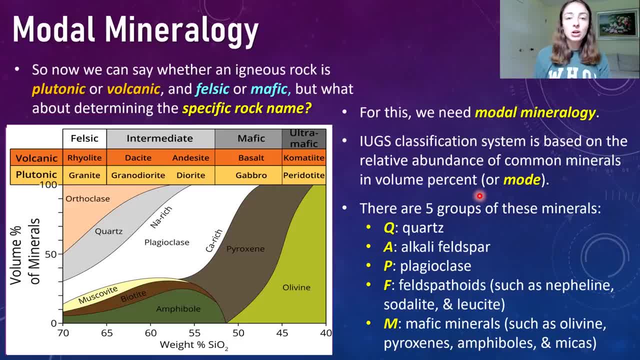 each mineral and determining the rock based on this relative composition that it has. so we can see in the description of this graph that the rock is based on this relative composition that it has. so we can see in this graph now that these minerals listed below the rock names on this graph of volume: percent of minerals. 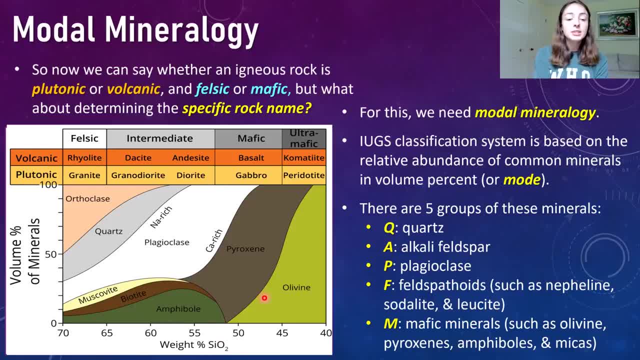 and weight percent of silica. on the bottom we can see these minerals plot in certain areas of the graph, which then determine the composition of these rocks, which then determines their name, and we'll show you the actual iugs classification diagram on the next slide. but before we do we need 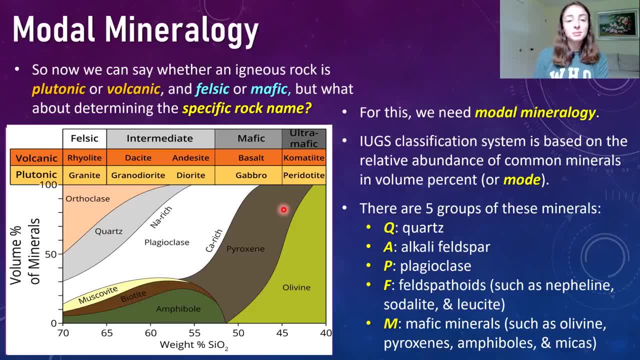 to talk about five major groups that the common igneous minerals fall under, because these are what the iugs classification system uses to determine rock names. what we can see is that these five groups include q, a, p, f and n. q stands for quartz, a stands for alkali feldspar, so alpha. 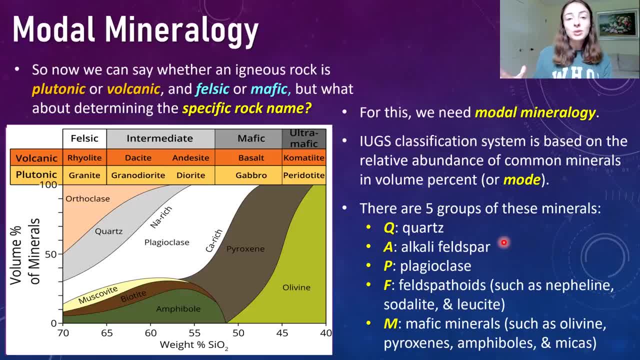 labeled spar is just on the more potassium and sodium-rich feldspar side of the feldspar spectrum and plagioclase, or p, is on the more calcium-rich side of the feldspar spectrum and you may think that isn't alibi technically similar to this. incredibly, ustedes decreasing al baわy-technguntaí. 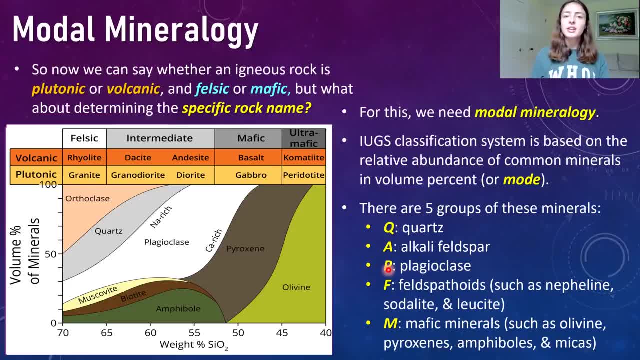 in the plagioclase feldspar solid solution series and doesn't it contain sodium? and so why is it included in alkali feldspar rather than plagioclase here? well, it's just how this classification system works. when we say p in this next diagram, that'll show you that means plagioclase on the anorthite. 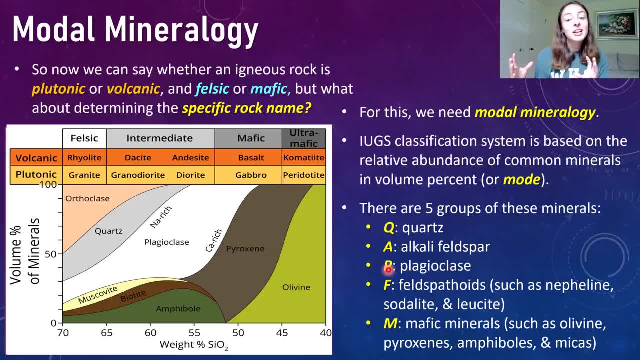 side, or calcium rich side, of the solid solution series plagioclase spectrum and not that on the albite side, which is the sodium rich side. actually that would indicate composition further toward the a side of the graph, which is the alkali feldspar side. so this will make more sense when i show you. 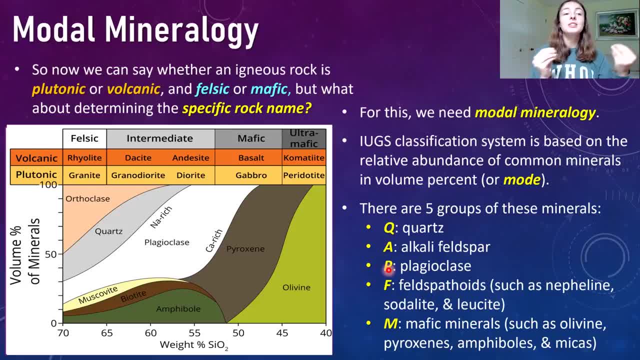 the diagram, but just know that sodium potassium rich feldspar is the a and calcium rich feldspar is the p. then we have f, which is feldspathoids, and i mentioned this word earlier. if you don't know what feldspathoid means, it's just minerals such as nepheline, sodalite and lucite. and last, 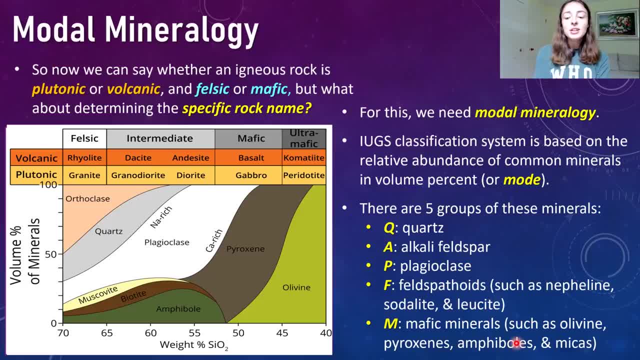 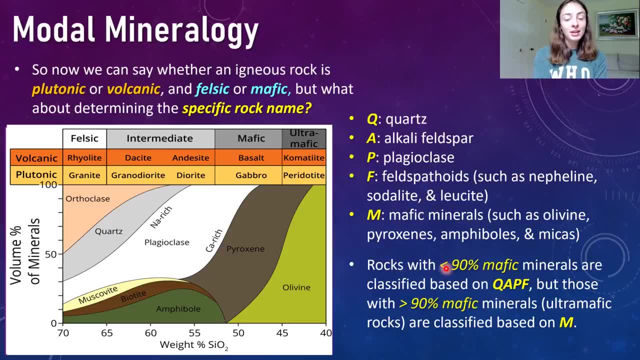 we have m, which stands for mafic minerals- so that's pretty easy to remember- such as olivine, peroxines, amphiboles and micas. rocks that contain less than 90 m or mafic minerals are classified based on just qapf and rocks that. 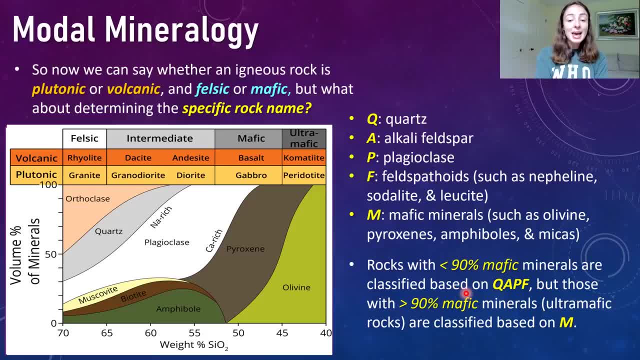 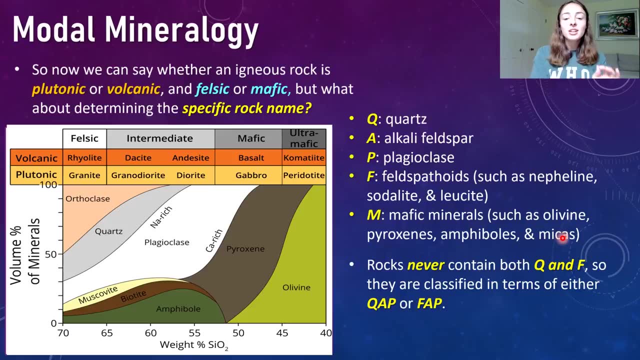 contain over 90 mafic minerals, or over 90 m, are classified just based on those minerals, and these tend to be ultramafic rocks. both felsic and mafic rocks tend to be classified using the qapf system. but before we look at the diagram, one more thing to note on the qapf system is that rocks never 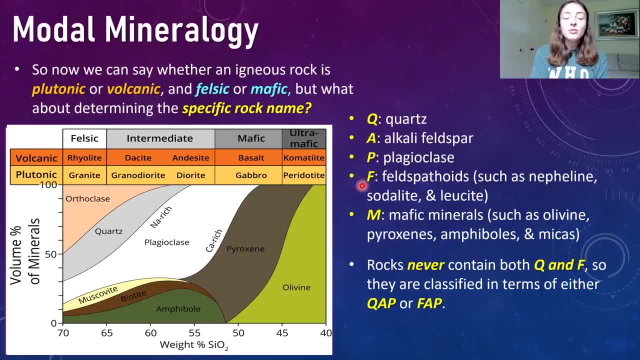 contain both q and f or both quartz and feldspathoids. don't get feldspathoids mixed up with feldspar, because they can contain both quartz and feldspar, but they cannot contain both quartz and feldspathoids. if you watch the rest of this igneous petrology playlist, you'll see me talk about phase diagrams in one of. 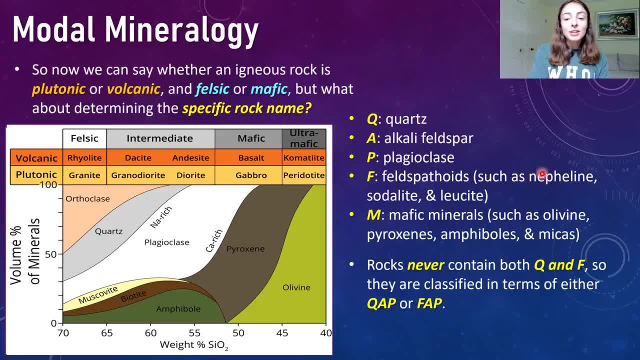 the videos, and there we'll talk about why minerals like nepheline and quartz can't crystallize together, and so don't worry about it right now. we'll go over that in that video. but basically they can't contain both q and f, so the igneous rocks classified using this diagram are: 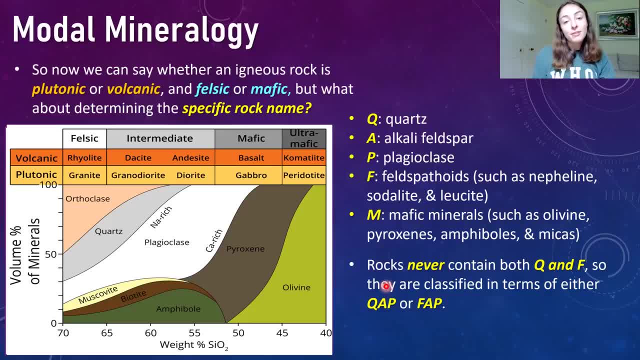 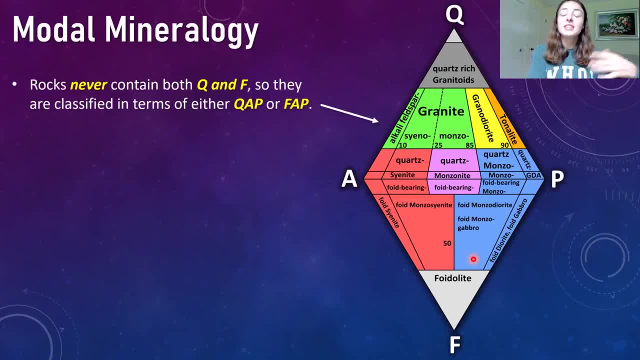 classified in terms of either qap or fap. we can see this on the qapf diagram. finally, we're looking at the iugs classification diagram of qapf. this is where we can classify felsic and mafic rocks and actually figure out their name based on their modal mineralogy. so basically a reminder: q is 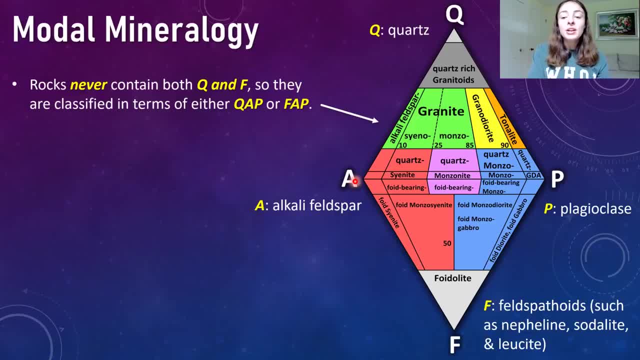 quartz f is felt, spithoids a is alkali, feldspar p is plagioclase, and the general plot of this diagram is that if you go up, you're increasing your quartz content or q or silica, and if you go down, you're increasing in belts with void content, which can also be thought as decreasing in silica. 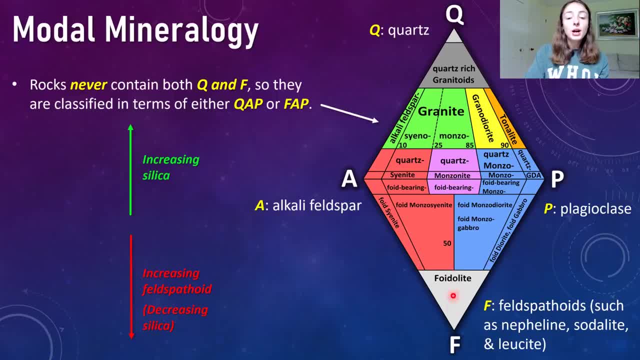 especially at this top half of the graph. once you get to the bottom half of the graph you've run out of q to decrease in and so you're just increasing in belts with void content. then, in terms of our a, we can see that going to the left is increasing in sodium and potassium. 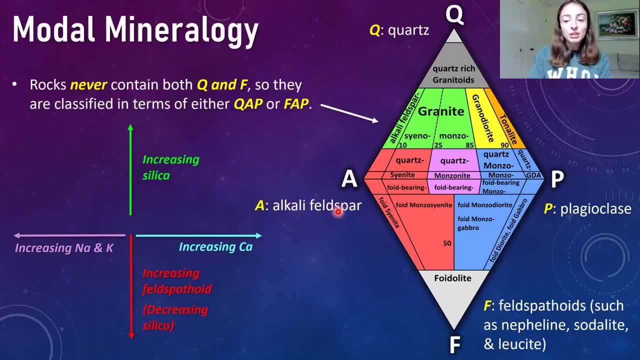 rich belts more, and going to the right is increasing in calcium rich feldspar or plagioclase, and so to define our y-axis, it's basically based on silicon content and our x is basically based on feldspar composition. now that we know how to read the 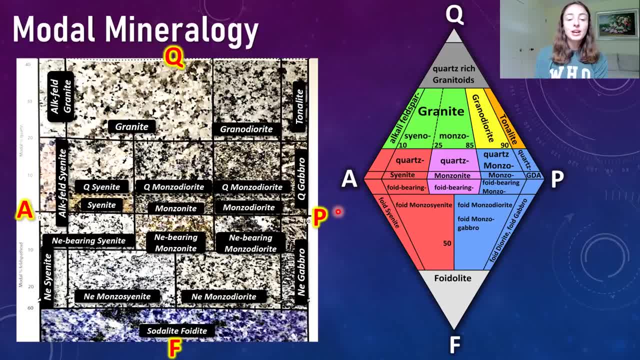 graph. i also want to show you this equivalent graph to the left here, where we can see this diamond graph laid out with pictures of each rock type. and it's all the same rock types and they're in the same configuration, with q at the top, f at the bottom, a at the left and p at the right. 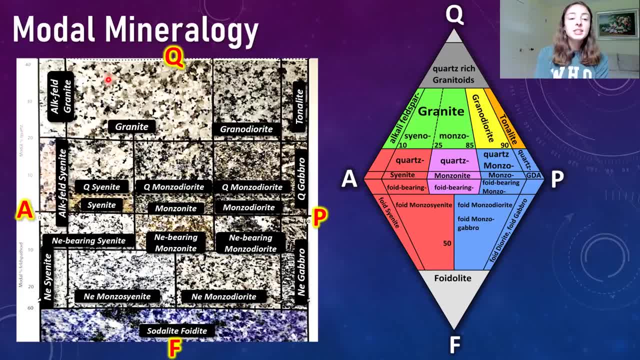 but they're on this square and we're showing pictures of the rocks. we can see that granite is relatively rich in q and can be rich in a or cyanogranite, and also can be in between a and p, called monza granite, and then we can also have 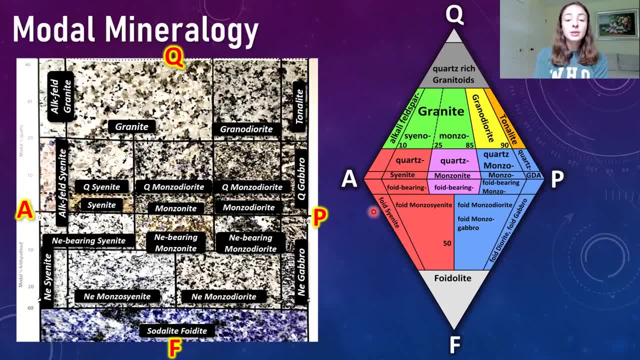 a really alkali feldspar rich granite or a rich granite called alkali feldspar granite. and then we can see that granite diorite is closer to the p side, so calcium rich plagioclase. we can see that in the graph to the left as well. and then we get to tonal light, which is 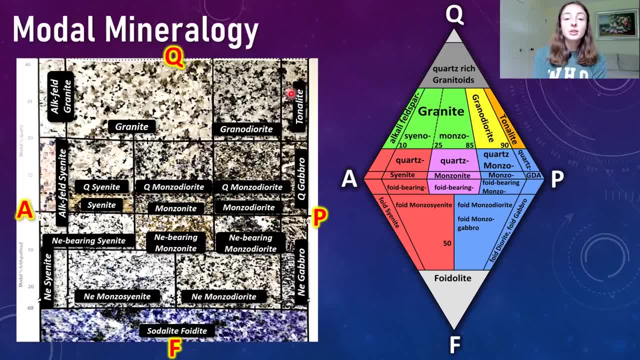 this orange field over here and also shown on the graph to the left as well, and it is also relatively q or quartz rich and very calcium plagioclase rich and hardly contains any alkali feldsparts. and then, if we go below the granites and toward the center of the diagram, we see that 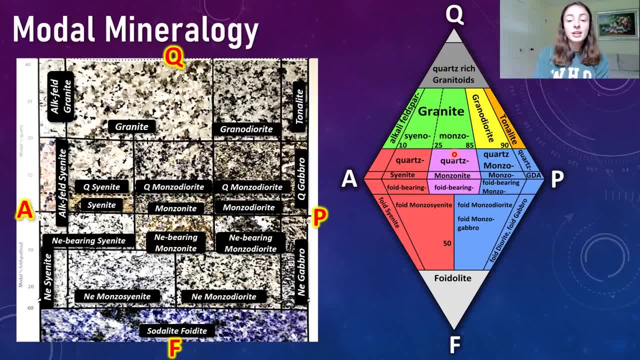 we have these prefixes here. so quartz cyanide, quartz monza night. we can see these in the picture to the left as well. that's what these q stands for: quartz cyanide, quartz bonds, quartz monzo diorite, so monzo diorite as well. and then quartz gabbro, and we're seeing: 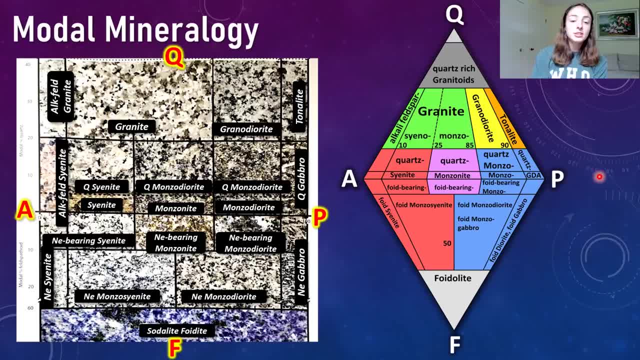 more mafic rocks here, because we know that the calcium rich plagioclase minerals are on the mafic mineral spectrum, whereas the alkali feldspars are felsic. we can also see that they're lighter in color, so this makes sense. more felsic minerals on this side are lighter. 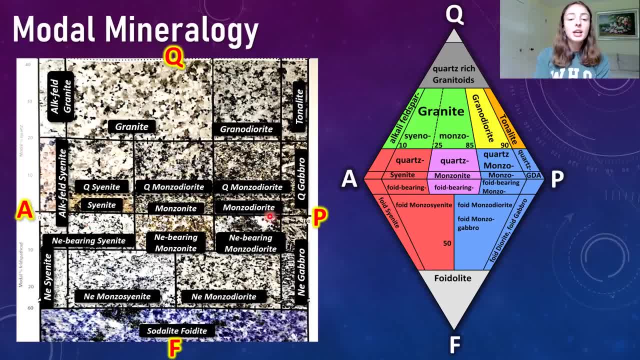 in color and more mafic. on this side are darker in color. and then we have these same minerals below quartz, cyanide and monza diorite, and these are just the same but without the quartz prefix. so we've got cyanide, monzonite and monza diorite. and then we have alkali feldspar cyanide, just. 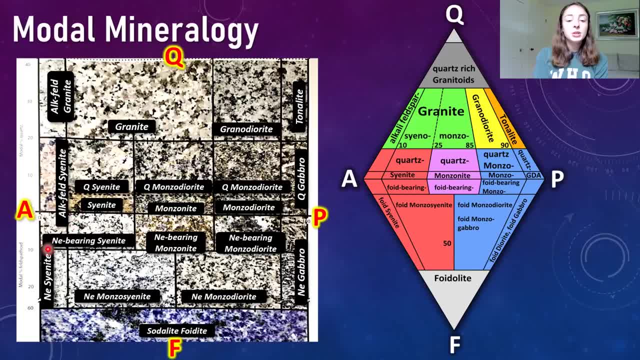 as we had alkali feldspar granite up here and then, as we move down below this barrier line that we cannot go between, we can only cross on either side. this marks the transition to feldspathoids, rather than q or quartz, and the feldspathoid transition. 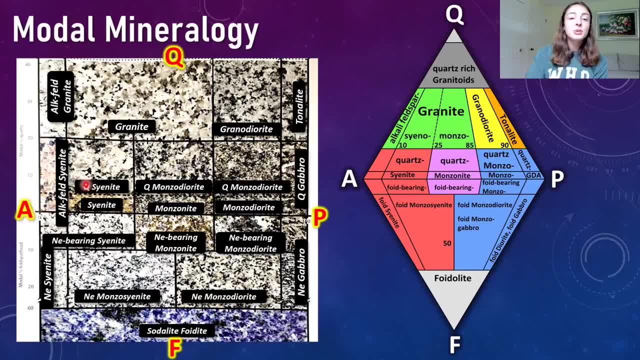 actually changes everything from being quartz whatever to nephilim whatever, and that's what the ne stands for. that stands for nephilim, and we can see that up here near the top, where you're not that rich in feldspathoids yet you're seeing it's called nephilim bearing cyanide or nephilim bearing. 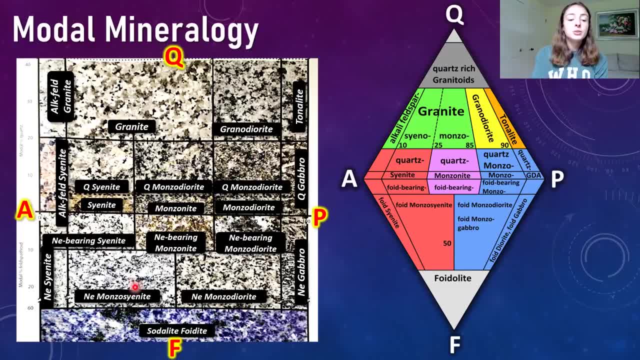 monzonite and monza diorite, but then you don't get to the nephilim monza diorite or nephilim monza cyanide until you get below that where you don't have to say bearing anymore because it's more rich. 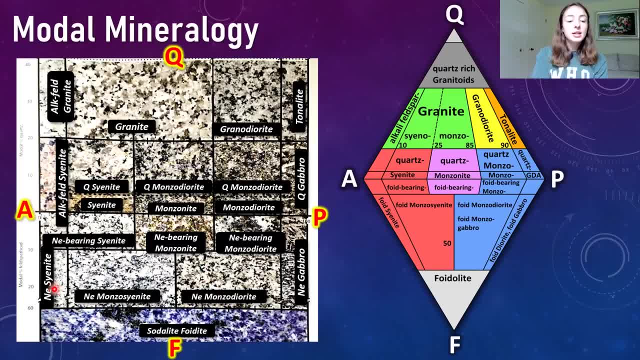 in feldspathoid than it is in feldspathoid. so that's why we put the mineral name in the prefix, and you can see this with nephilim cyanide as well and nephilim gabbro on the mormaphic side or p side. 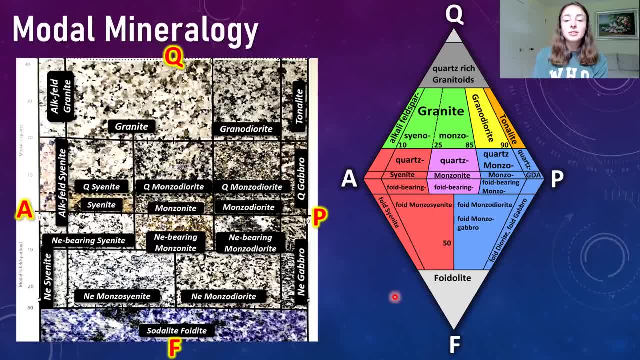 of the graph to the right and then lastly, at the bottom, we have sodalite fordite. that's also shown on the diamond diagram over here. we also see that this diamond diagram does not specify that the feldspathoid bearing rocks in these red and blue and purple regions are nephilim, but instead just: 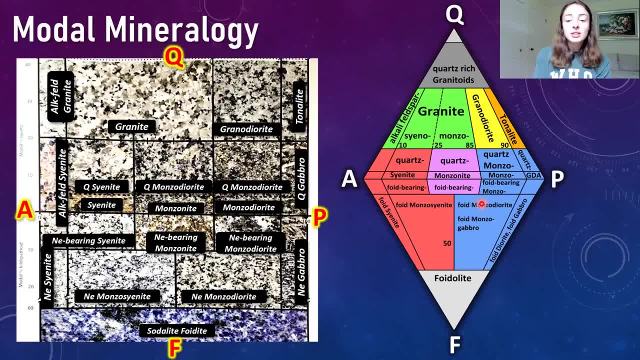 says void, to keep it general, because there are other feldspathoids that are not nephilim. but nephilim is a mineral that is not the only feldspathoid mineral that can be bared in these rocks just below the ap line, and that's why foydolite is called foydolite, because it has so much feldspathoid. 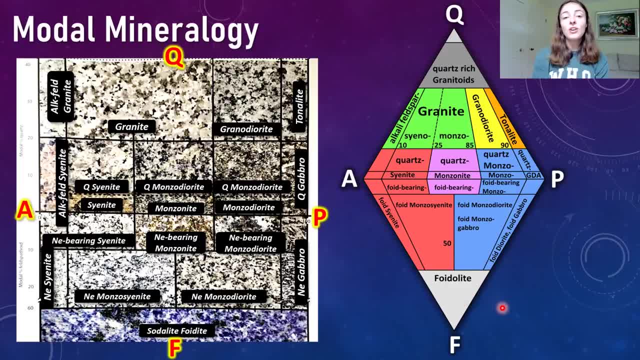 or foid for short, that it is just almost all feldspathoid and so it's called foydolite and can also be really rich and so delight, and so you can put that mineral name in front of it and that's also a general rule, as you can tell, throughout these entire decades of mineral. 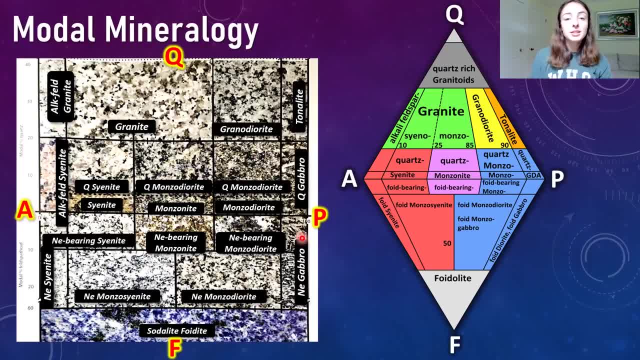 diagrams that the mineral that might be most abundant in that rock tends to be put in front of the rock name and that's pretty common if you want to specify what you're looking at. if you're not totally sure and you just see a felsic rock that you can tell has alkali feldspars, it has. 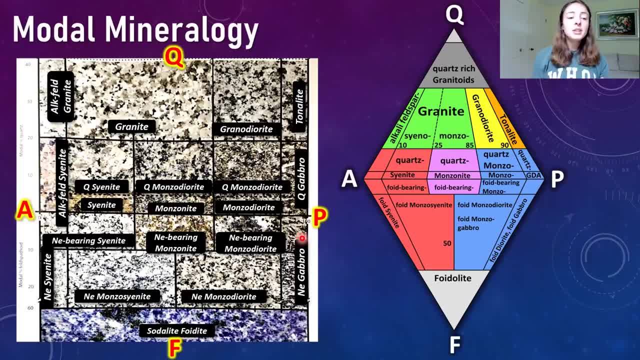 quartz, it's coarse grained, you can just say granite. but if you think it's so rich in alkali feldspar, or potassium feldspar specifically, that it's turning pink- because typically case bar rich granites tend to turn pink- you can say it's an alkali feldspar granite or a case bar. 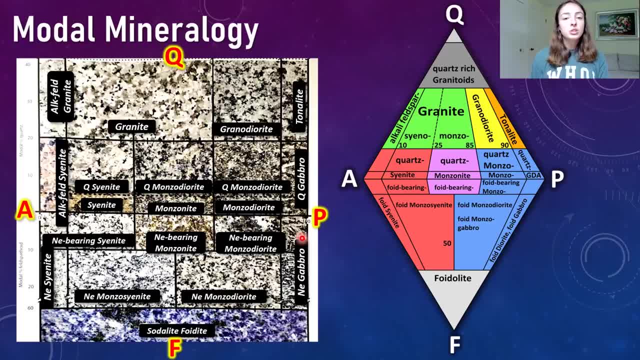 granite, because you're being more specific with that name rather than just calling it granite. however, you can also go to the other side of the spectrum with, say, gabbro. you can tell that you have a dark mavic rock and it's coarse grain. so you know it's gabbro, but if you think it has a 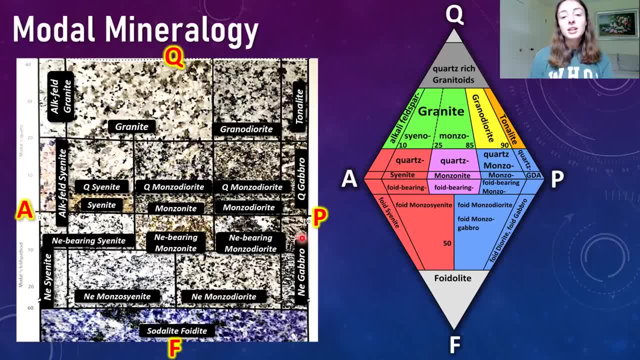 rich amount of quartz in it or a rich amount of nepheline in it. you can call it quartz gabbro or nepheline gabbro to specify further its mineral content. and you can also go to the other side of astrology without being so vague, and the rule of thumb is to put the most abundant mineral right in. 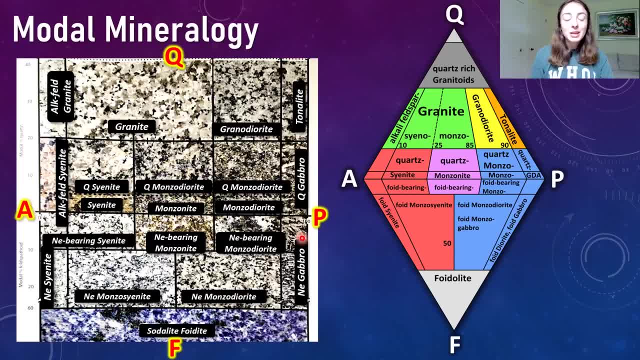 front of the rock name. for example, if you think there are two major mineral constituents in your gabbro, such as biotite and hornblende, and you think the hornblende is slightly more abundant than the biotite or much more abundant, you can call it biotite hornblende gabbro, but you can't. 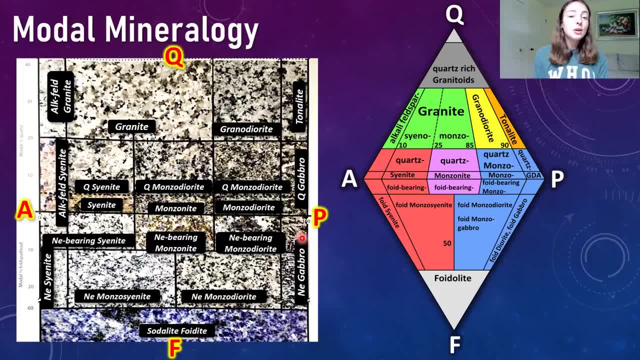 call it hornblende- biotite gabbro, because you have to put the more abundant mineral name right in front of the rock name. so it would be biotite- hornblende- gabbro. but you can't call it hornblende, biotite hornblende- gabbro. or if it had more biotite, you could put biotite right in front of. 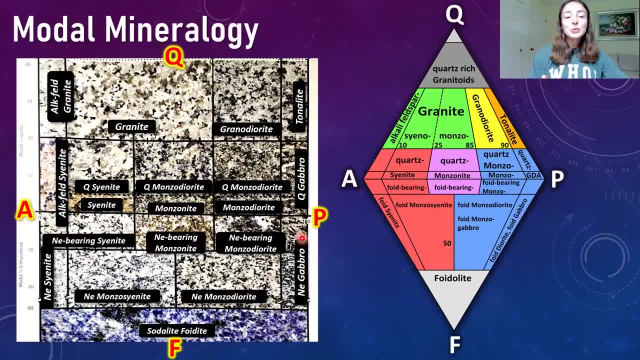 the rock name would be horrible, biotite gabbro, and so, anyway, we're getting too far into it. i think in terms of classes, you'll be fine just knowing granite or gabbro and you don't need to know all the specific minerals that you can put in front of the name. but it depends on your professors. 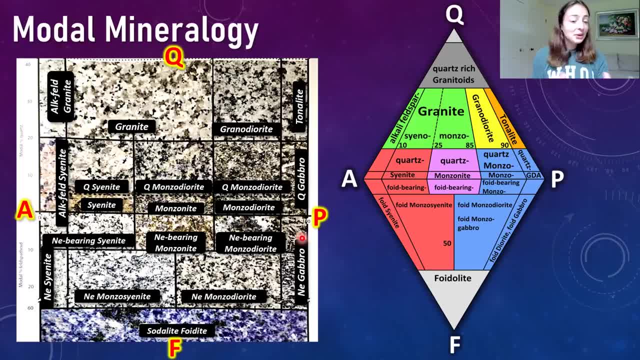 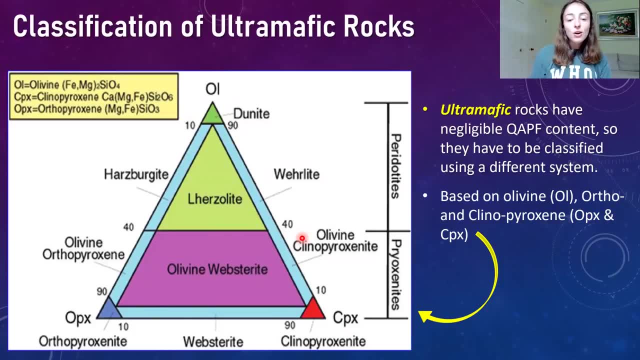 and what they are wanting from you. so now you know how you can do that if you have to, but also know that you know keeping it broad if you're not sure what the most funded minerals are is better than trying to guess and getting that wrong. so, like we mentioned earlier, ultramafic rocks have over 90 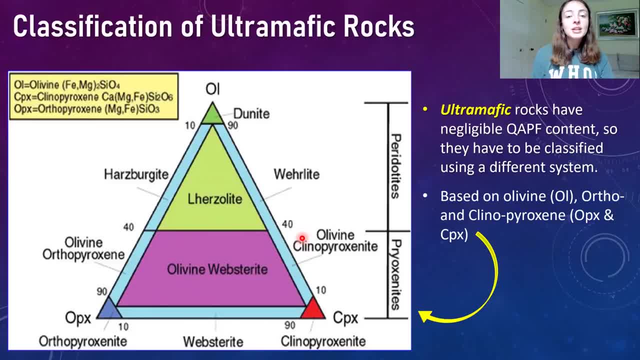 mafic minerals or m, out of our qapf m categories. and we know that the qapf diagram cannot classify ultramafic minerals because they have to be classified based on their m contents or their mafic mineral abundances. and so how we do, 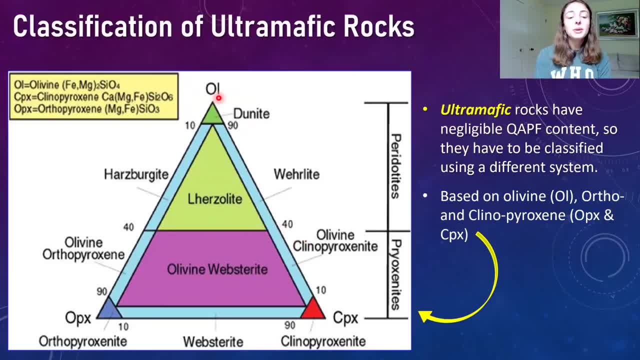 this is using this triangle diagram here, where we have mafic minerals on each corner of the triangle, so we have olivine at the top and then peroxenes at the bottom, and the left bottom corner specifically is orthopiroxene, a specific type of peroxene, and the right bottom corner is clinoperoxene. 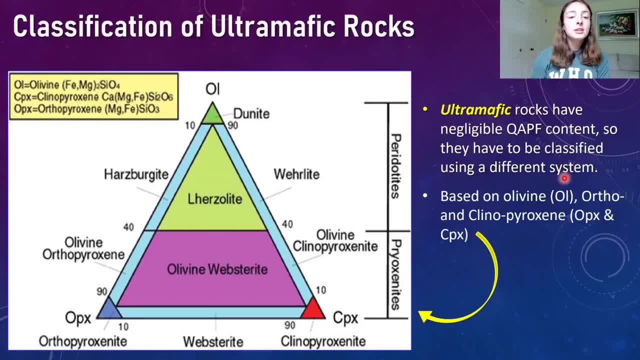 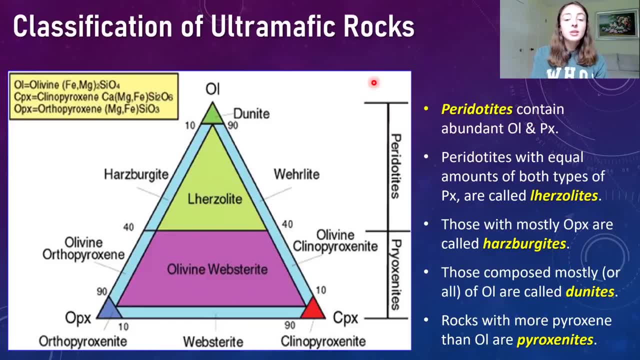 and so this ultramafic rock classification system is based on these three minerals, and we can see that peridotites contain both olivine and peroxene, so they fall into this top half of the triangle graph because they contain olivine and peroxenes. 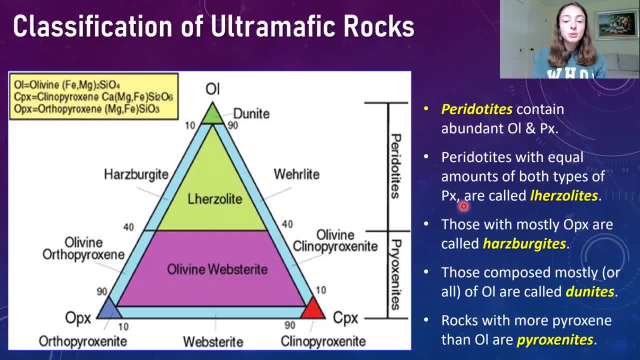 and peridotites with equal amounts of both types of peroxene so that fall in the middle of this upper half of the triangle fall under layers of light. so layers of light is a rock that has both clino and orthopiroxene and also abundant olivine, and it is a peridotite, but it's more. 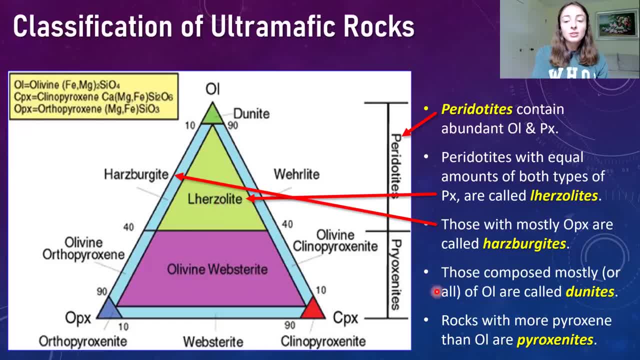 specifically layers of light, peridotite, and then you have the last one, the pyridotite, and then you have the pyridotite and the pyridotite. that are both different. the pyridotites and the have those that contain mostly orthoperoxines, and these are harzbergites, harzbergites, yeah. 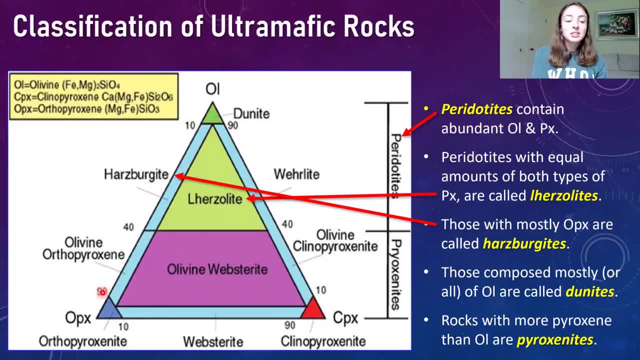 harzbergites on the very left side here. that's because it's mostly orthoperoxine. also has olivine. it is a peridotite, but it doesn't have enough clino peroxine to be in the larizolite range. 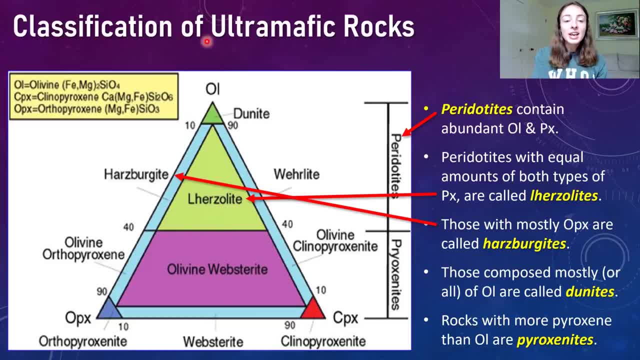 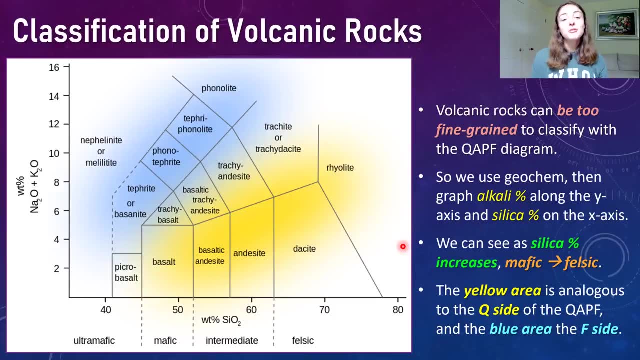 so it's harzbergite. and then we can see those that contain mostly olivine are called dunite. and then the bottom half of our graph- here we have those that have more peroxine than olivine, and these are peroxinites. so you've probably noticed throughout this lecture that we've 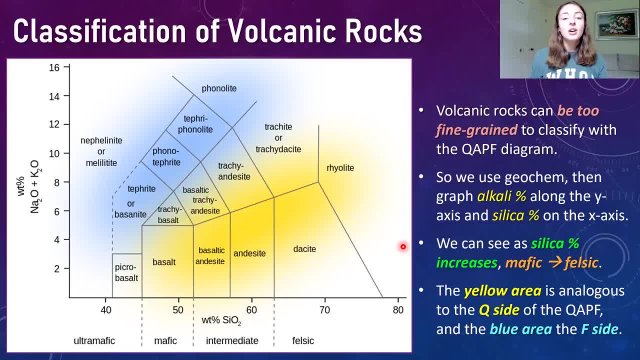 been able to classify felsic and mafic plutonic rocks on our qapf diagram and ultramafic rocks on the diagram on the previous slide. however, what about those two fine grained to be classified using the qapf diagram? this tends to happen with volcanic rocks because, as we know, 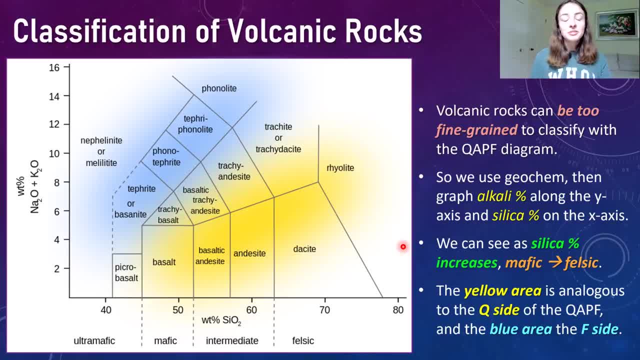 volcanic rocks can have very fine grains because they explode out volcano and they cool very quickly and they don't have time to grow large grains and therefore we have to have this other system to classify volcanic rocks. this system, also made by the iugs, uses geochemistry of the rocks, so 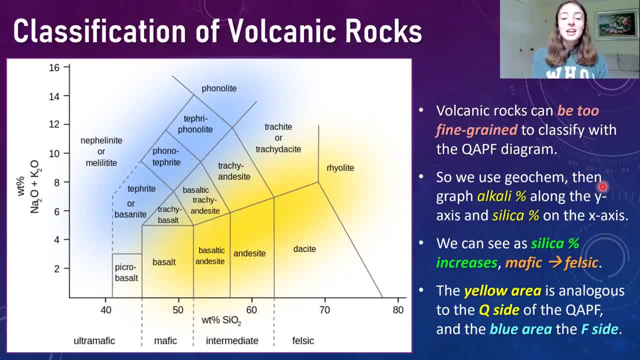 geochemical composition, by geochemical analysis, and what we use is alkali percentage, so alkali weight percent or sodium and potassium weight percent along the y-axis and silica weight percentage along the x-axis. and so what we see is that silica percent increases as ultramafic goes to mafic and intermediate and then felsic, finally with the highest. 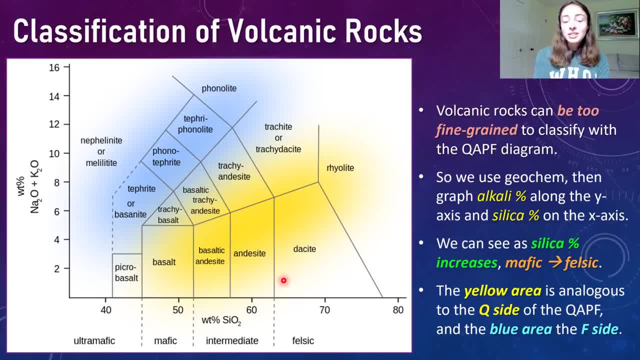 silica weight percentage. so this makes sense. and not only does it make sense, it also follows along our qapf diagram pretty closely. actually, we can see regions of this diagram in yellow and blue, and what these represent is the q side of our qapf diagram for the yellow region. 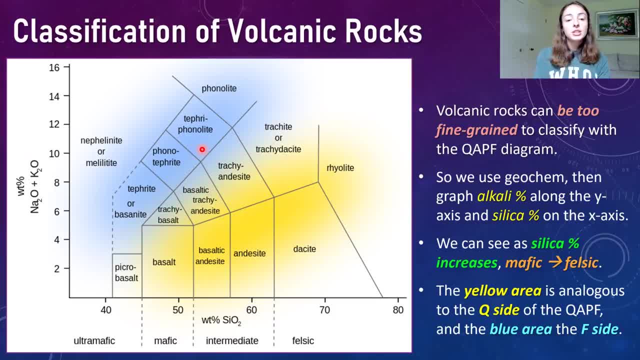 and the f side or feldspathoid side for the blue region. so it's pretty similar to what we have in our qapf diagram and we can now see that these rock names all correspond with volcanic rock equivalents of what we saw in our qapf diagram. for example, on the q side of things, the yellow, 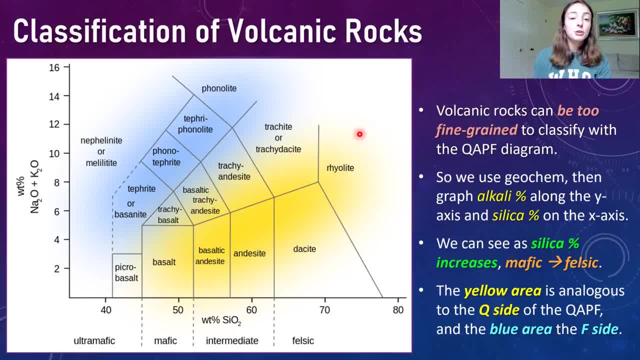 region we get rhyolite, which is our granite volcanic equivalent. so granite is the plutonic or coarse-grained version of rhyolite, and so we have rhyolite in this q or yellow region of this classification system. then we have daysite and andesite as intermediates, and these are volcanic. 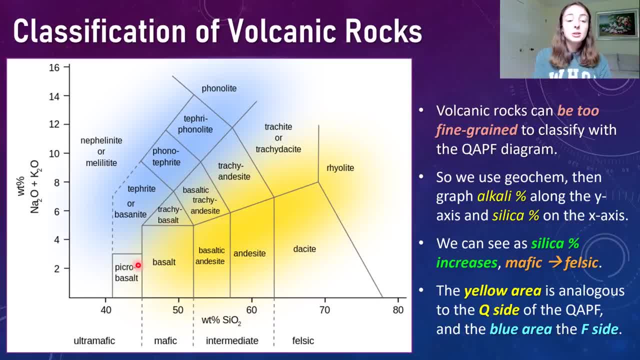 equivalents of diorite and granite diorite. and then we move to the basaltic range, where we have basalt, which is the volcanic equivalent of gabbro. and so now we can almost see that not only is the yellow region the q region and the blue the f region, with our feldspathoid rich equivalent of the q region. 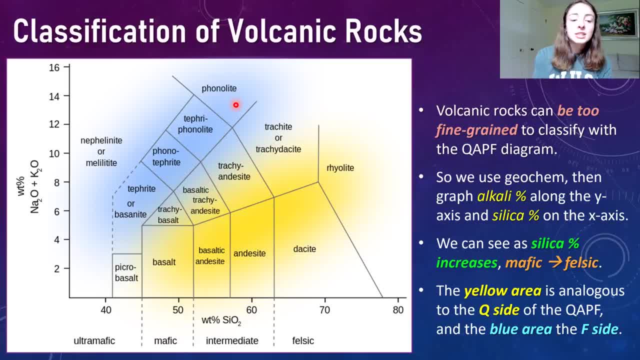 so nepheline rich rocks over here, we can also see that basalt is over here and rhyolite is over here, and so this is probably more mafic, as we can see with these labels, and this side is probably more felsic, and with that we can kind of make it equivalent to our diamond graph and say, oh so. 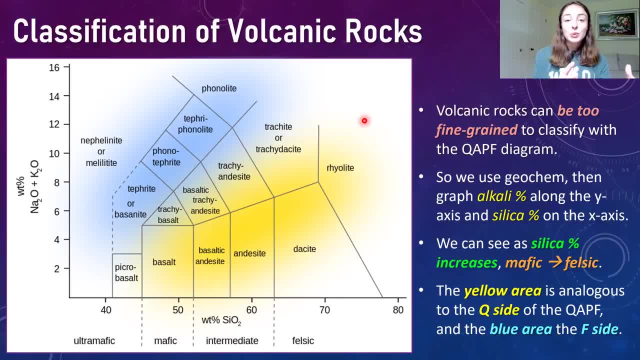 this more felsic side is probably the side that we saw the granite on on the diamond graph, so the more a or alkali rich side, whereas this side down here with much less alkali feldspar content is probably on the more p side of our diamond diagram, and so i'm not going to talk about all. 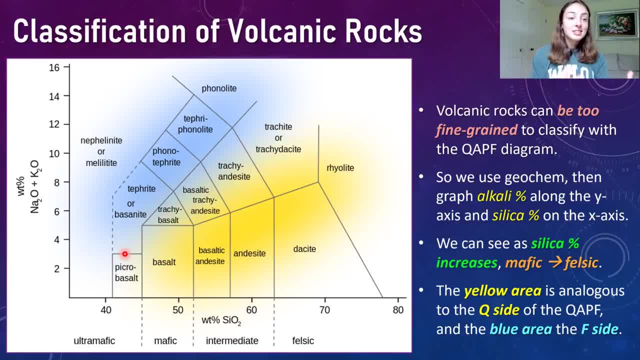 rock names. you probably get the general trends on this graph, as it is the same as the general trends on the previous diagram, just instead of plutonic rock names these are now volcanic rock names, which are different than plutonic rock names, but for every plutonic rock there is generally a volcanic 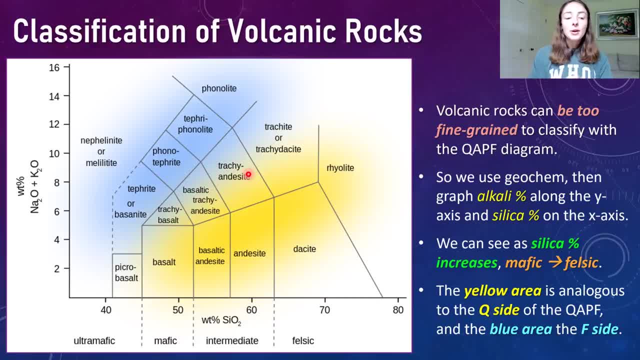 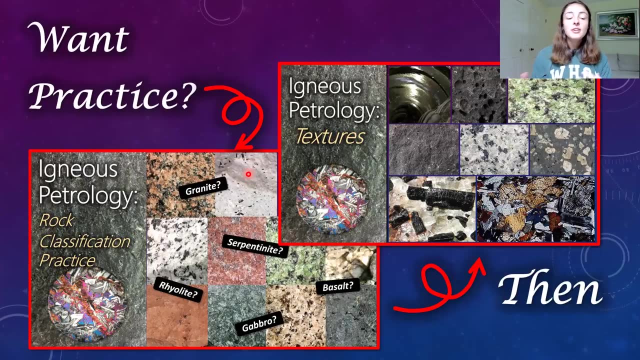 equivalent or fine-grained equivalent rock. however, there are exceptions in the ultramathic world because ultramathic rocks form weirdly, but we'll talk about that in an upcoming video when we talk about igneous rock textures. so that is in the upcoming content. 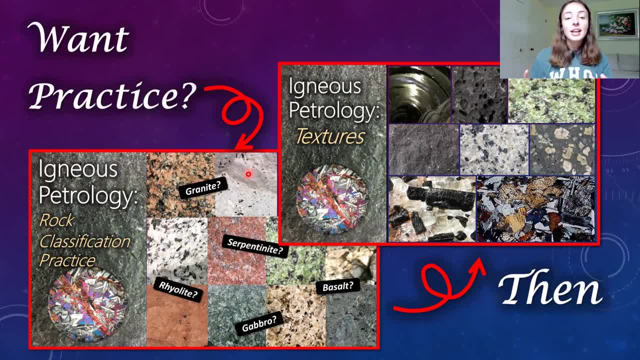 if you want practice identifying or classifying igneous rocks, don't worry, i have a separate video coming out as a part two kind of to this one, in which we'll classify igneous rocks based on their hand table pictures. maybe some thin sections i'll throw in. 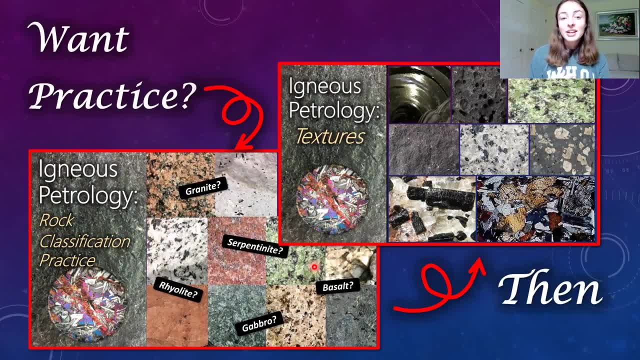 there as well, and we can do that now that we have our basic knowledge of these classification systems. so we'll do that in the next video and then after that, like i mentioned a couple times in this lecture, we'll talk about igneous rock textures. so we've got glassy, we've got vesicular, we've got pegmatetic.